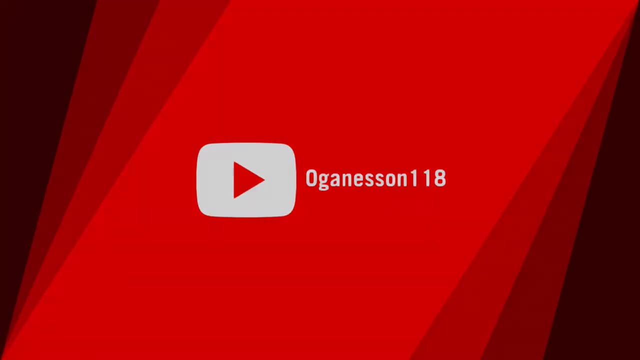 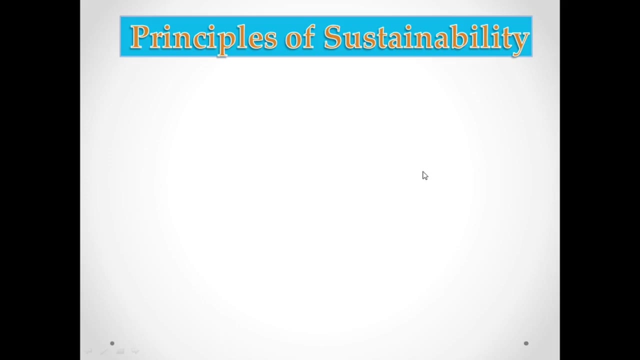 Now let's move to our next topic, which is the principles of sustainability. There are actually three principles of sustainability, and life on earth has been sustained billions of years ago because of these three principles. Number one is the dependence of solar energy. Number two is 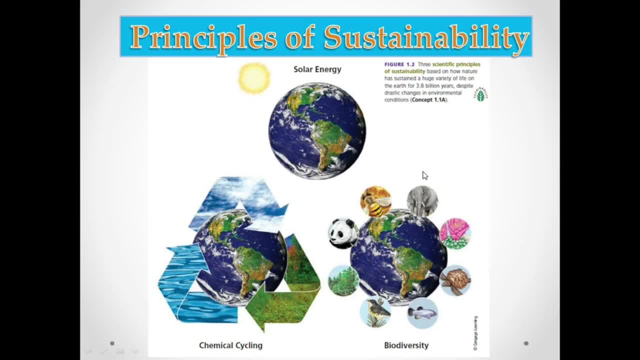 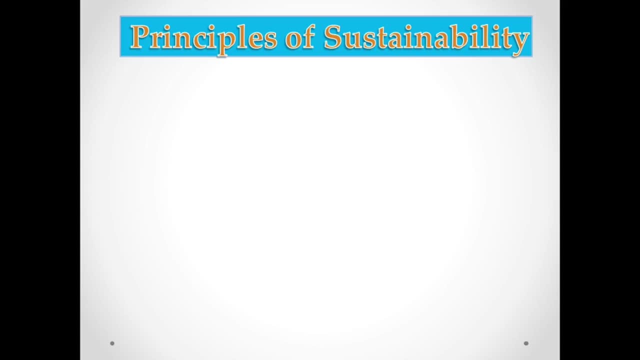 chemical cycling. and the last one is biodiversity. First, we're going to talk about the dependence on solar energy. So the dependence on solar energy is that sun inputs solar energy to warm the planet. okay, it warms the planet and provides energy that plants use to produce nutrients. So we have learned this during our 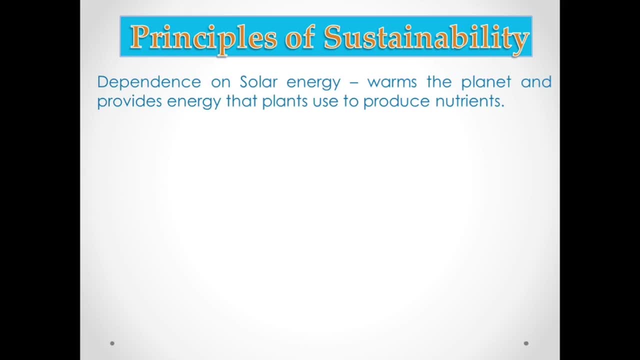 elementary days that this is what we call the photosynthesis. okay, So the photosynthesis is actually the food producing process of plants in order for the plants to grow, to survive and reproduce. okay, and because of this, if the plants are reproduced and also grow and produce its own food, those animals that depends on plants will also survive and grow. 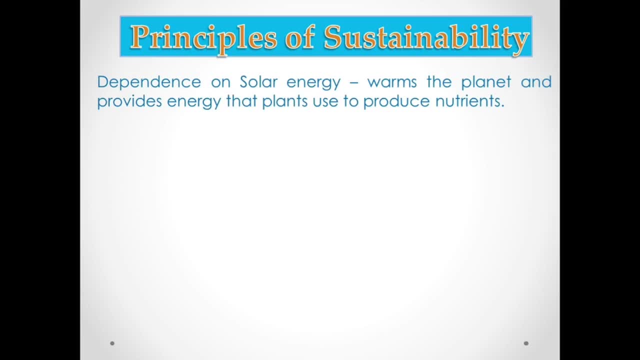 develop and also multiply on the set of on that environment where it exists. okay, and because animals also depends on the plant, okay, we also, humans, also depend on the plants, because we also get our resources or our food and in plants. okay, and also some of the things. 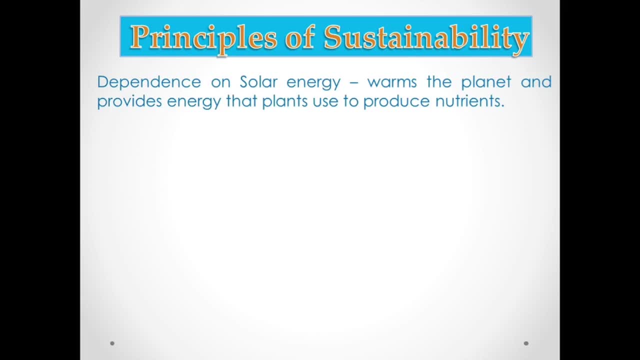 that that we need, we all. it's also coming from plants, coming from trees or in the environment, and also the animals get a meat, okay, and the animals okay. so that's it. so we depend actually on the solar energy. So that solar energy, okay, we survive because, uh, because of those factors that I actually mentioned earlier, and not just that, okay, solar energy is also important because nowadays we have a, we have a solar panel, okay, which which uses solar energy to produce electricity. okay, so that is how solar energy is very important and without it we can't survive. 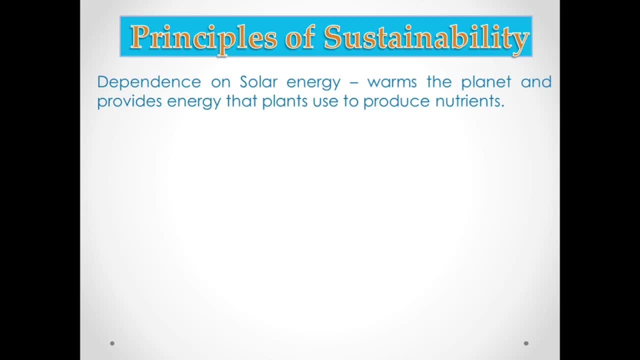 with the planet and modified science. and, more importantly, we can never survive. okay, We can never survive. okay, we can never survive. buy, it's something that you, you need the economy to survive. and number two Cause you can only survive by, you can't survive and we can never survive. 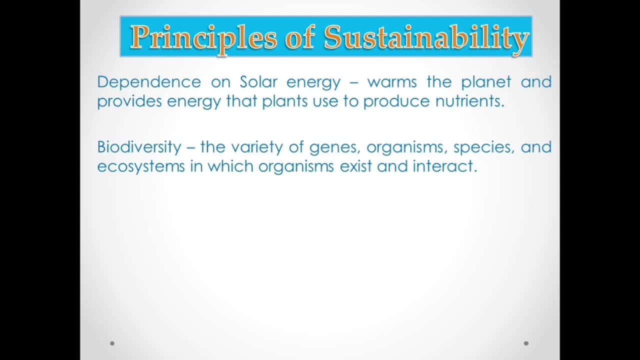 Okay, And number 2 is biodiversity. so biodiversity is a short or biological diversity. it's actually the variety of genes, organisms and species and Ecosystems In which organism exists and Enter up, exist and interact, but it also studies the of how these organisms actually have. 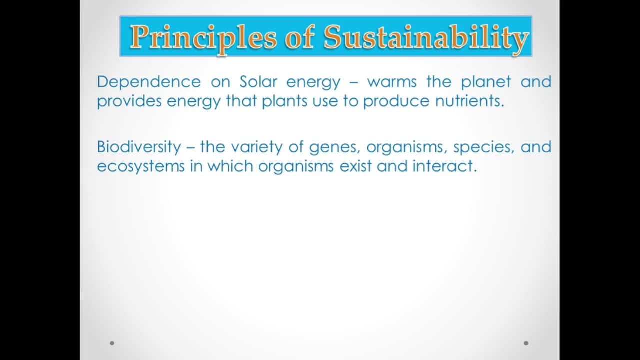 a feeding relationship or how are they going to survive on that ecosystem or on that environment where they belong in or where they, where they are, actually exist or present there, okay. so so like, for example, we will also talk about in the biodiversity, we will also talk about food chain, okay, and also food web, okay. 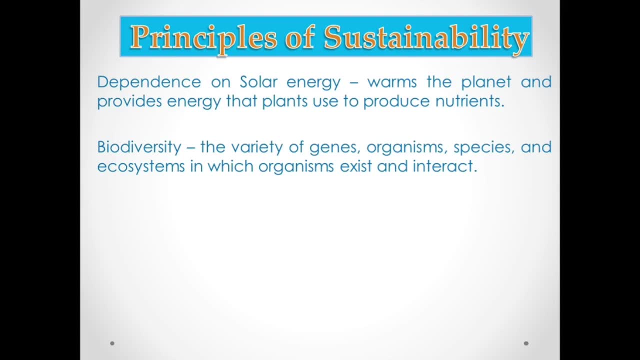 so we knew about food chain during our elementary or even in high school. okay, the consumer, the producer, a first-order consumer, then we have the. the last one is the decomposer- okay, and also the interconnecting food chain, which is what we call the food web. okay, so we will talk about that later on as we go to. 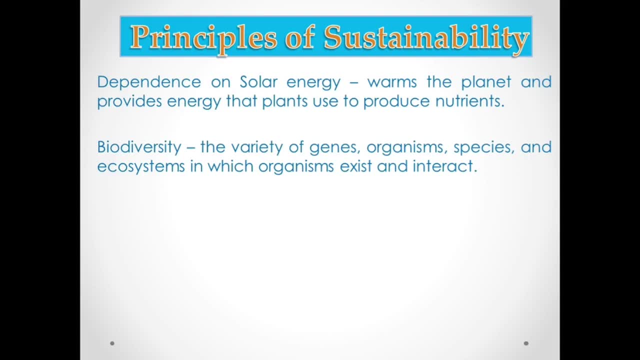 topic. okay, so we should, so that we can learn more on the, the interaction of the living organisms to the environment. okay, so that's it. that's the biodiversity. and also because of biodiversity, organisms have the ability to adapt the drastic condition or environmental changes and drastic conditions in the environment. 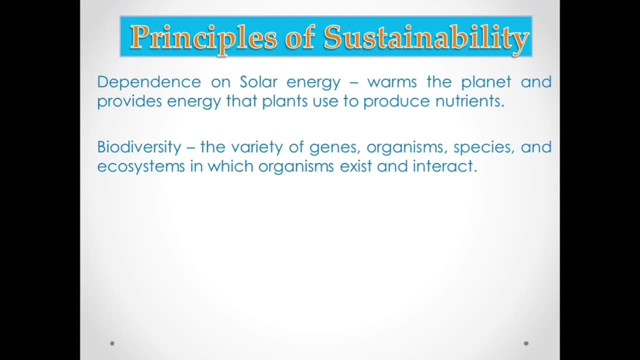 as well as environmental changes. okay, because of biodiversity, because there are a lot of variety of genes already. okay, from the offspring, of offspring of the parent. okay, so the the genes are already mixed. okay, from the father or the mother of that offspring. so, therefore, because of that, a variety of genes and 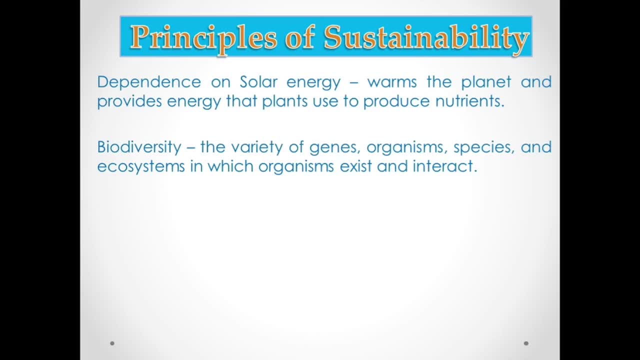 the possibility is that kind of species can adapt to the change in the environment or the drastic change of the environment. okay, and the last one is the chemical cycle. okay, so when you see chemical cycling, it's actually the circulation of the chemicals necessary for life from the environment to 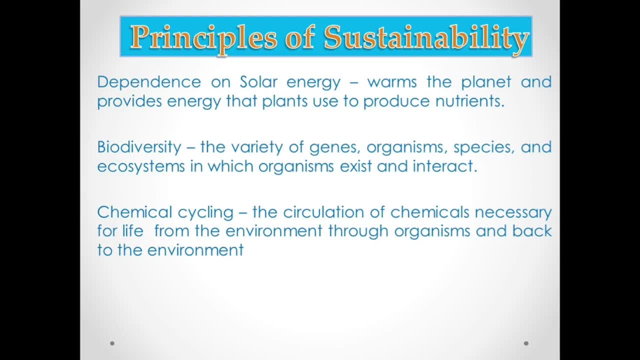 organisms and back to the environment. so chemical cycling is also called the nutrient cycle. so these are there: carbon cycle, the water cycle, okay, the phosphorous cycle, the sulfur cycle or the nitrogen cycle, and we will talk about that as we go through the chapter on the environmental science or this textbook that includes the topic. 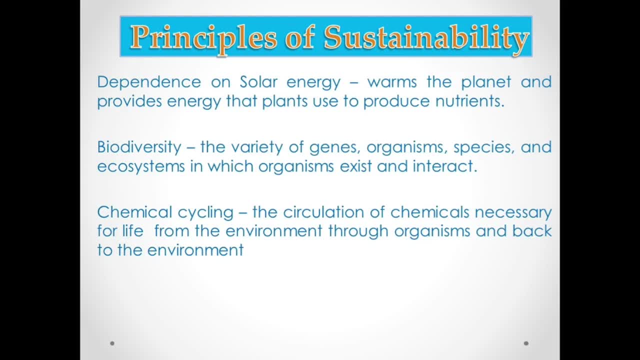 on chemical cyclings. so this chemical cycling is it's actually very important, okay, and and it's because in this question that has been shown in my Nigerian freneticlı fathers there were temperatures around 16°C on the 15-20°C warm when then blowing. 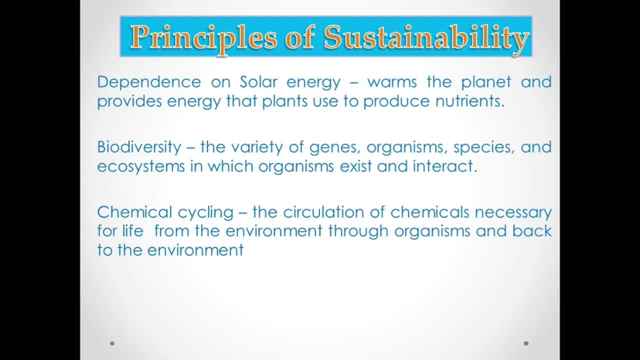 in nature or the environment, there are actually less uh waste. okay, it's actually not waste because, as when the when the organism, or when that species or when that organism dies or decompose, okay, it actually goes back to, to the soil and those uh chemicals or waste. 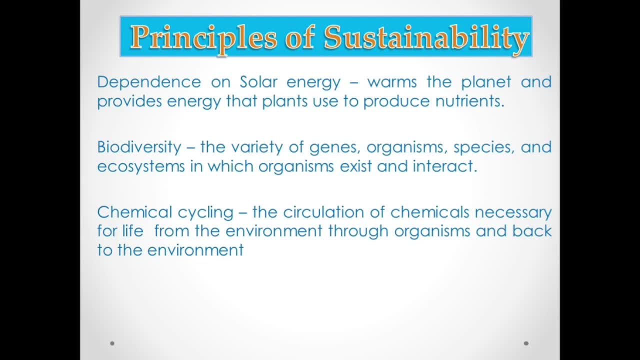 okay, that are actually, uh, in the soil will become a raw materials for, or a fertilizer, or a raw materials to for other, or for the plants to grow. okay, because that becomes a nutrient of the plants. okay, and therefore it actually recycles. okay, it actually recycles again. 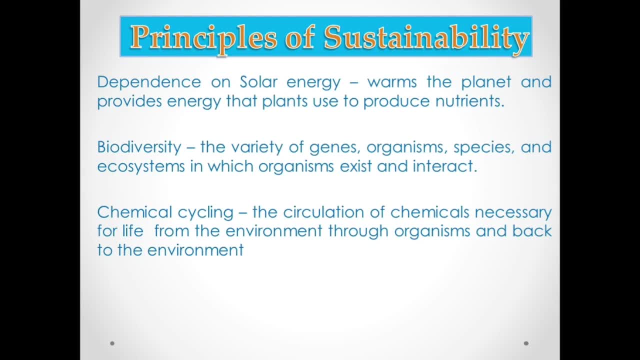 it will be used by the plants for it to grow, okay, and for it to grow, multiply the living animals, which those animals will eventually, uh, eat the plants and after that, when that animals dies, okay, it will be decomposed and those ways, okay, that the animals are produced. 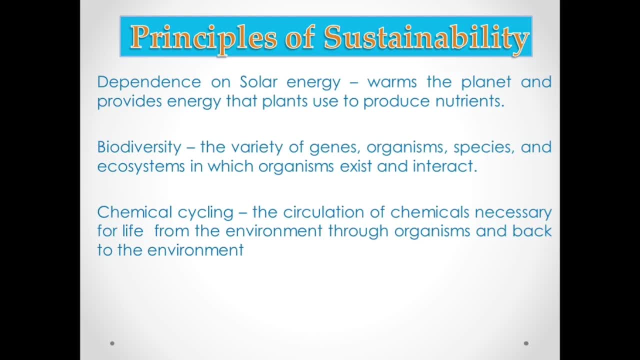 okay, will eventually use again by the plants, by the other plants. okay to be for that plants to multiply again. so as you can see in nature the ways there are actually useful resources. okay, so there are actually less ways in nature rather than in the human world. in nature the ways is.